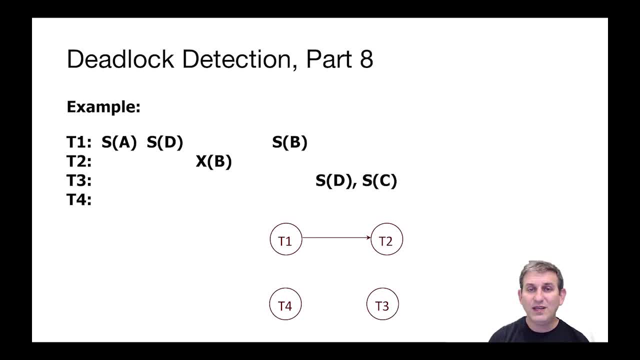 which it can share with T1, so that's fine. T3 now wants a shared lock on C, which it can get. T2 wants an exclusive lock on C, which means that T2 is going to be waiting for T3 that holds that shared lock on C. T4 can run still. T4 wants an exclusive lock. 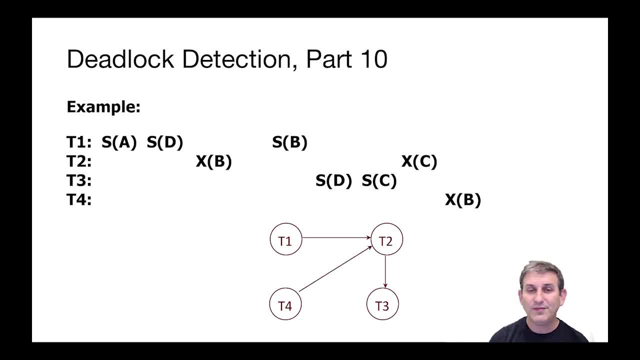 on B, which means that T4 is going to be waiting on T1,- excuse me- on T2.. T1 is also waiting on T2, right? They're both waiting because of that exclusive lock that T2 has on B And. 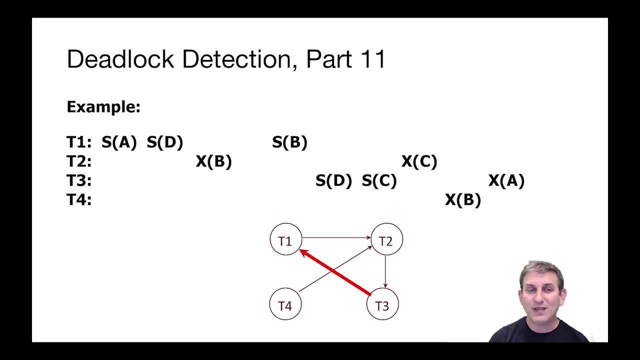 then finally, T3, which can still make progress here, decides it wants an exclusive lock on A, which makes it wait on T1. And I've colored that edge red because it's the edge that creates a cycle: T1 is waiting for T2,. 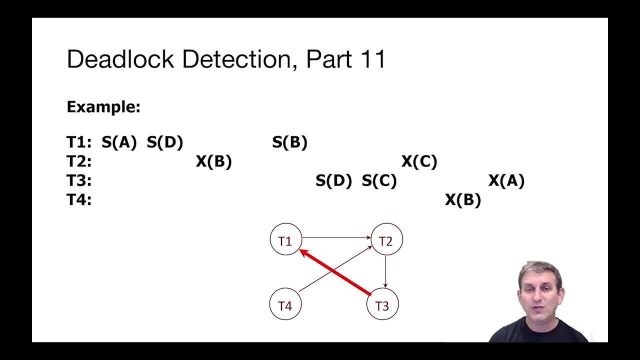 T2 is waiting for T3, and now T3 is waiting for T1, and we know we have a deadlock. So the deadlock detector is literally creating a graph of who waits for whom, so we can find cycles in the graph. A cycle in the waits for graph is a deadlock. 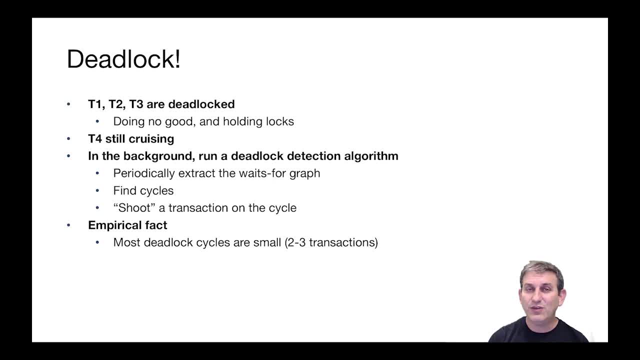 So when these things are deadlocked, they're doing no good, They're holding locks. Note that T4,, by the way, is still cruising along doing its work, So it's not like the system is useless, It's just not doing anything useful. 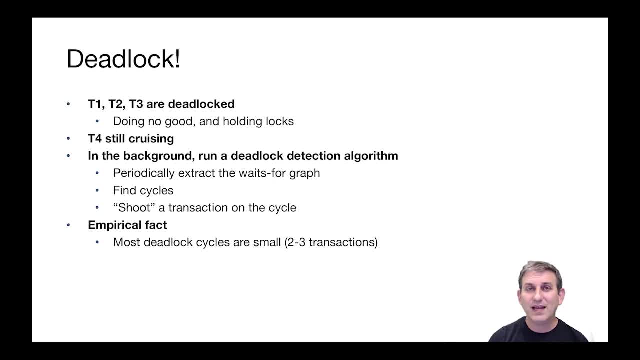 For T1,, T2, or T3.. And so in systems that do deadlock detection they just periodically in the background extract the waits for graph from the lock table, find cycles and they shoot a transaction on the cycle, which is to say they abort one of those transactions. 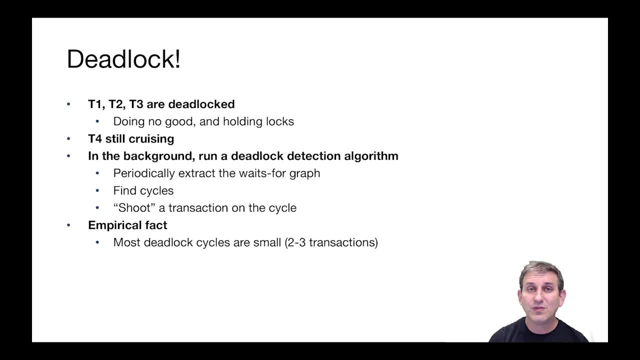 on the cycle And you could again abort the oldest transaction or use some sort of priority scheme to choose whom to abort. An empirical fact that's been seen in systems- and this has been studied quite often- is that most deadlock cycles you get are small. There may be two or three transactions around. 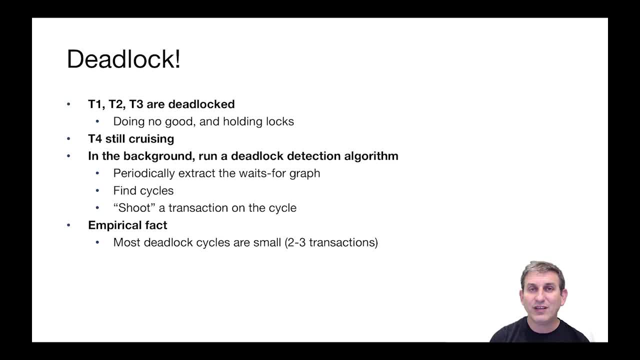 And so it's not difficult to find these cycles and it's not very costly to abort one transaction to make them go ahead. So deadlock detection and deadlock resolution where you kill one of the transactions in the cycle is very typical in most database systems that implement two-phase locking.